with respect to, which does causes sting. 1 1, N, up, 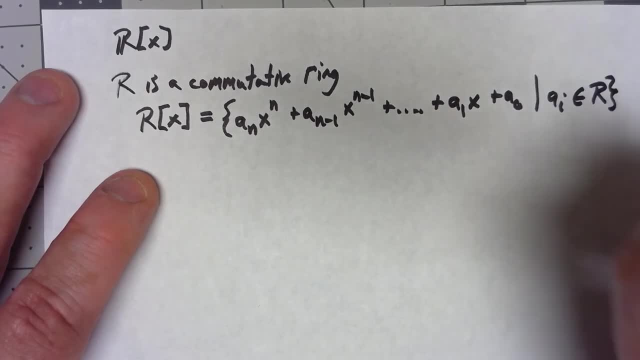 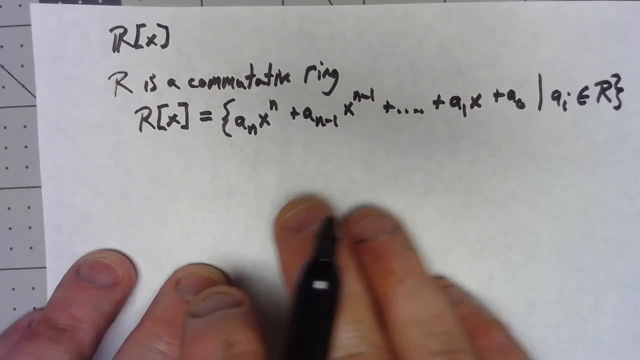 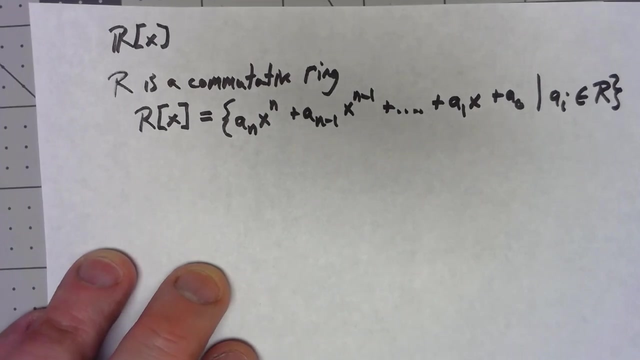 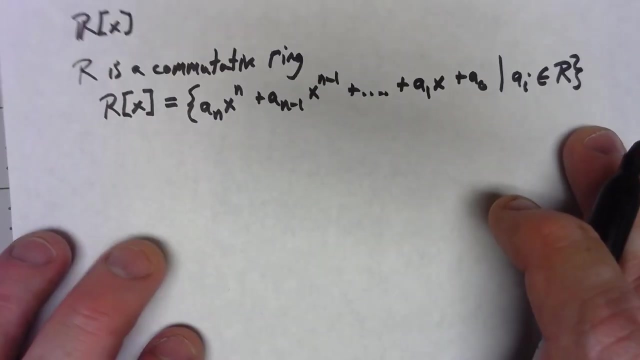 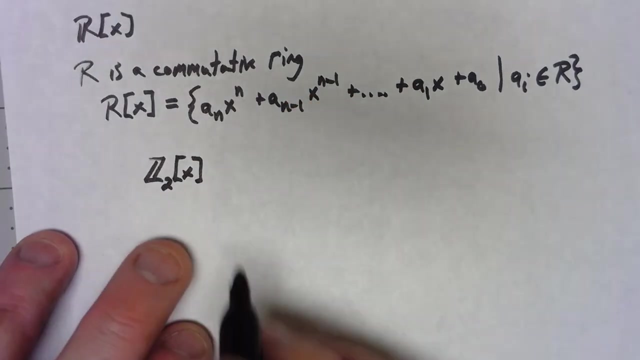 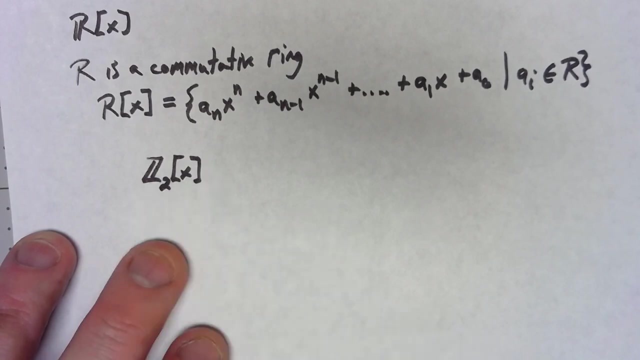 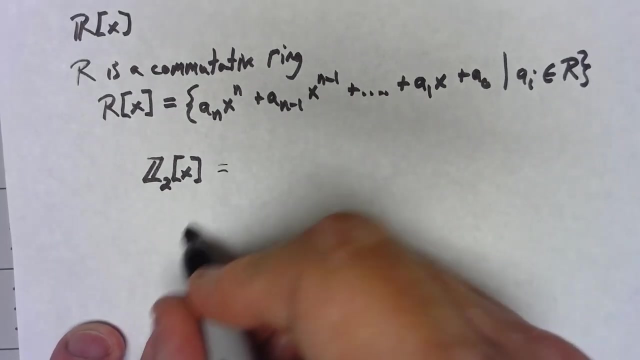 AIs come from our commutative ring. Now, if we do that, addition and multiplication in this thing are going to be exactly what you think they're going to be. Rather than trying to do it in general, let's take a look at a specific kind of thing. So, if I have z2 x, that's going to be the set of all polynomials like this, where our coefficients are either 0 or 1, because they have to come from z2. So, I might have something like an element of that is x cubed plus x squared plus 1. 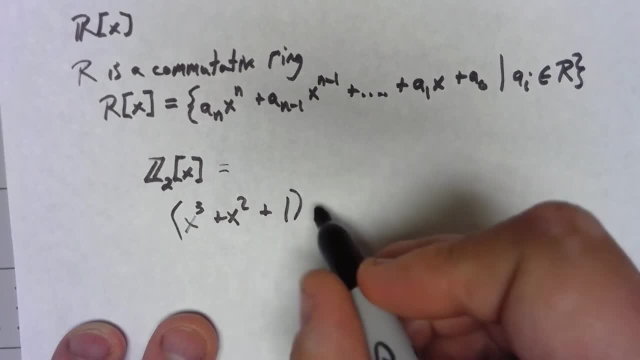 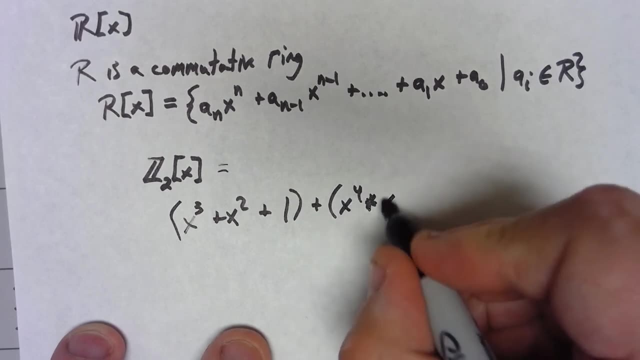 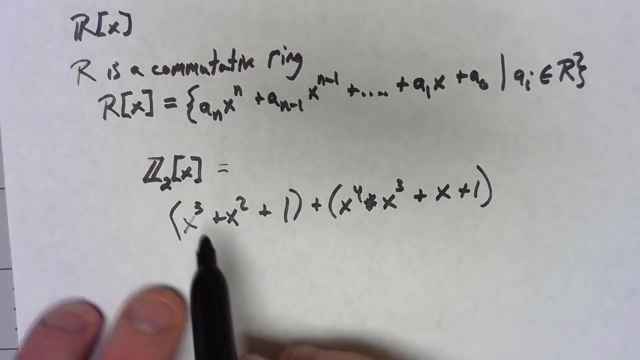 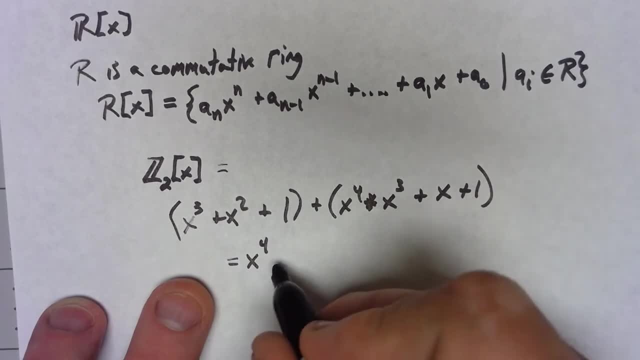 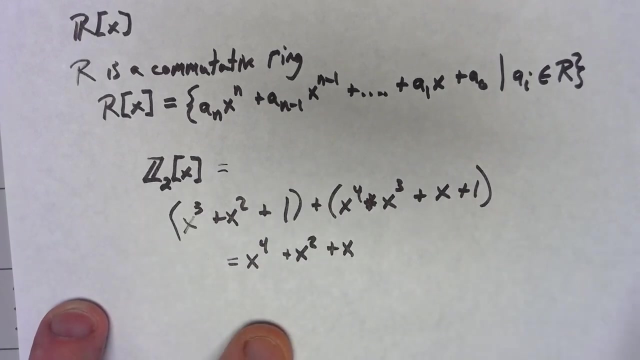 cubed, that's 2x cubed, but mod 2, that's 0. That comes out. We only have a single x squared. We only have a single x. When I do 1 plus 1, I'm adding in z2. So, I get just x. 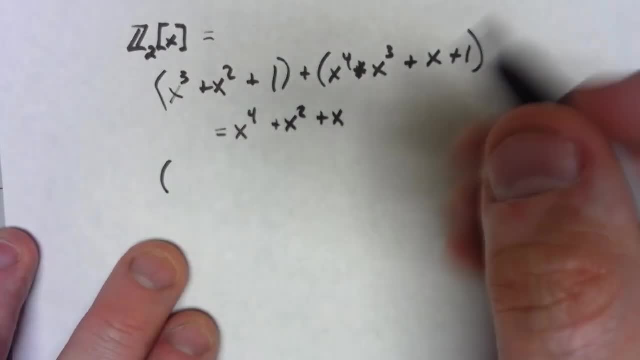 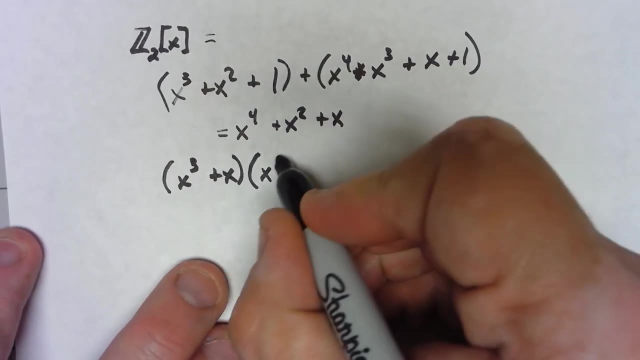 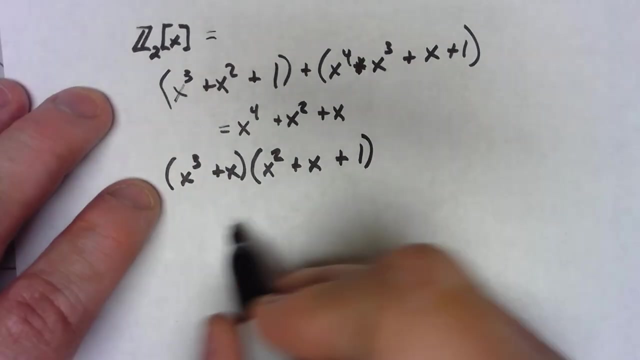 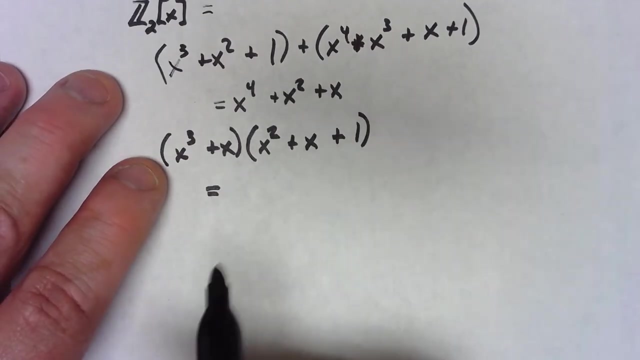 Similarly, if I have something like x cubed plus x, and I'm going to times it by x squared plus x plus 1, I'm going to basically foil it out just like you would a normal thing. So, we're going to have x 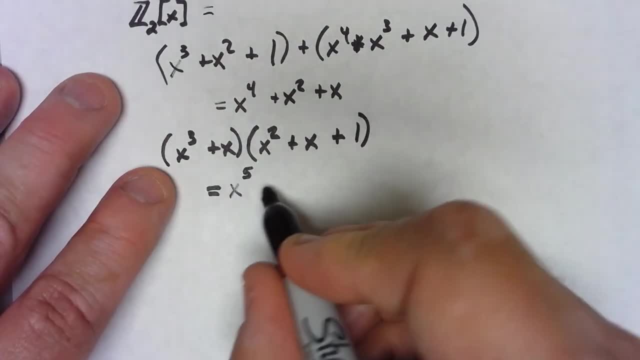 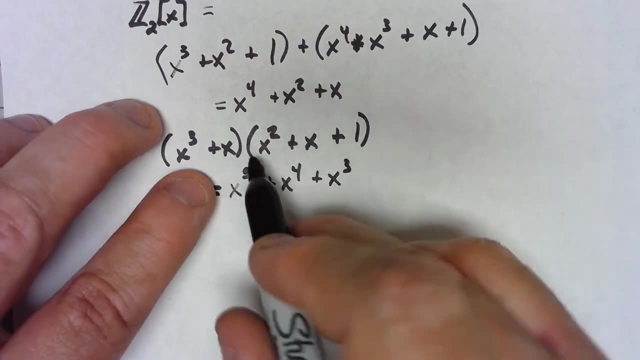 cubed times x squared is x to the fifth. x cubed times x gives me x to the fourth. x cubed times 1 gives me x cubed. x times x squared is x to the fifth. x cubed times x gives me x to the fourth. 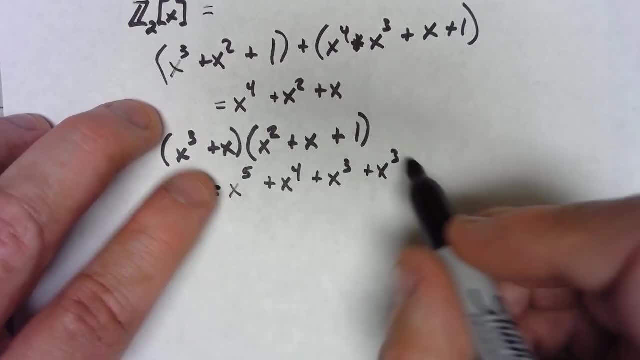 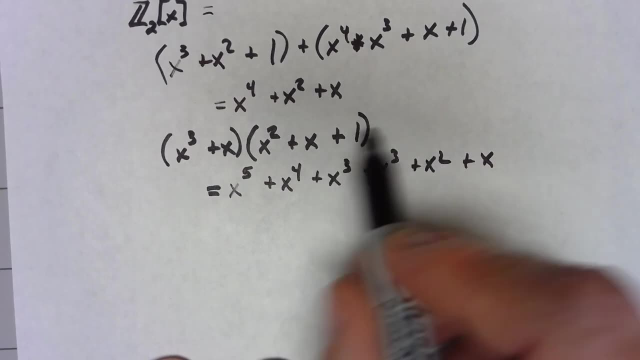 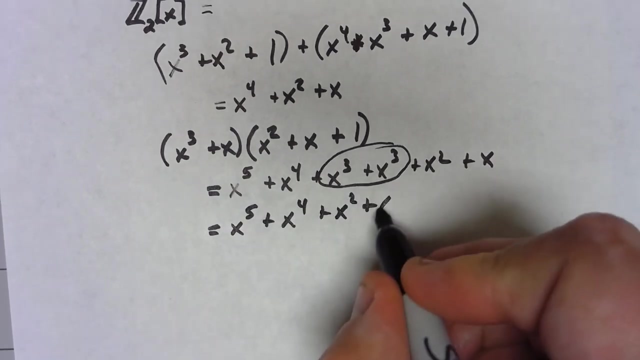 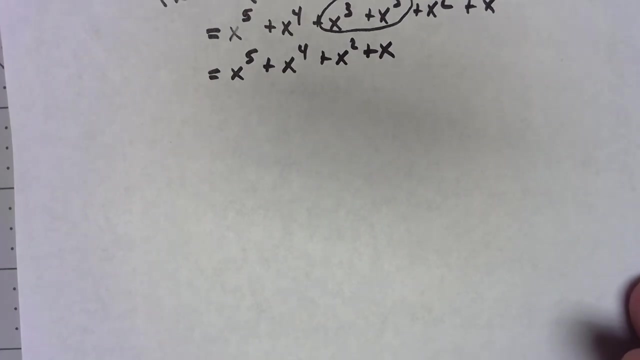 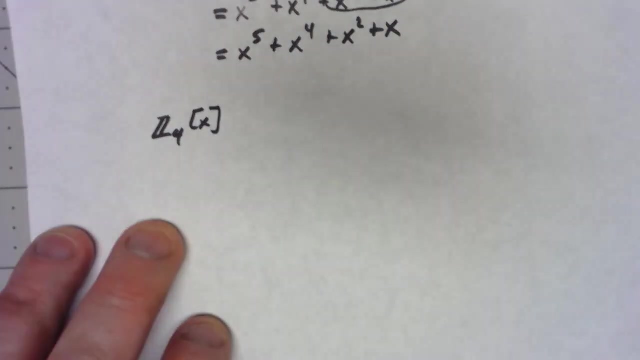 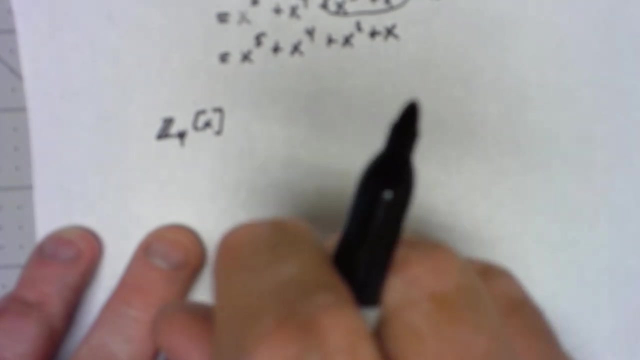 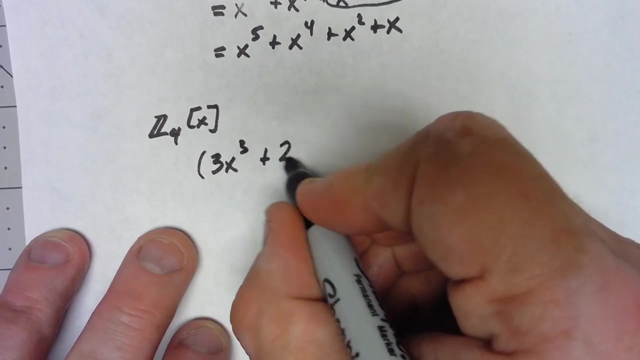 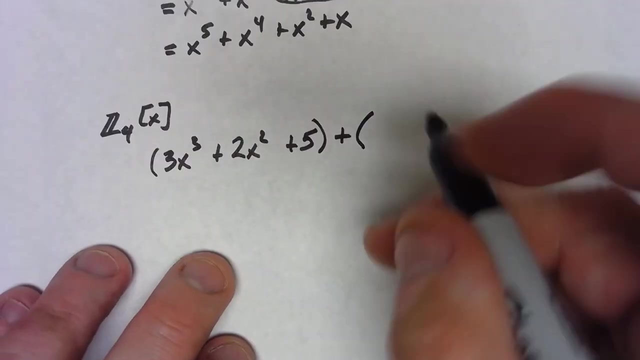 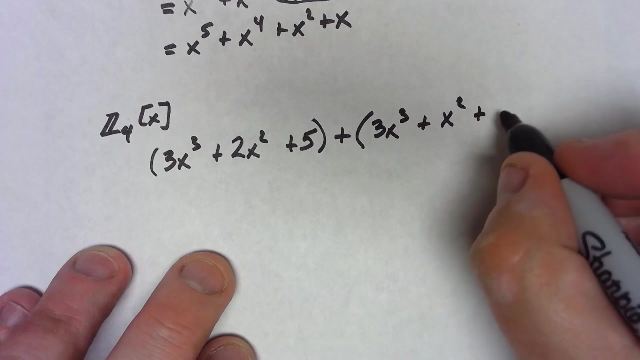 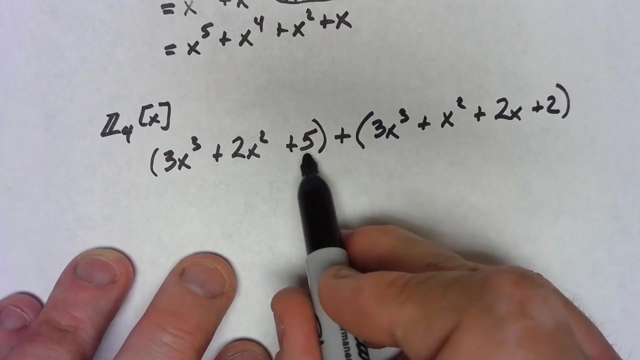 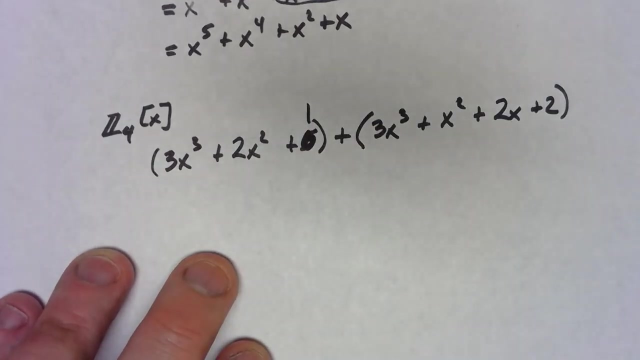 x squared gives me another x cubed. x times x gives me an x squared. x times 1 gives me an x. And then when I combine like terms, once again, I'm adding them, taking the coefficients in z2. So, x cubed plus x cubed is going to give me 0. And this thing is x to the fifth plus x to the fourth plus x squared plus x. Let's do it again. And let's maybe go to, say, z4x. Just to, so we've got things that aren't just binary. So, now my coefficients for my polynomial can be either 0, 1, 2, or 3. So, let's say I have something like 3x cubed plus 2x. Let's take that. So we get 3x squared plus 5. And if I add 3x cubed plus x squared plus 2x plus 2, and actually, hold on, I said plus 5. That doesn't exist in z4x. I can do plus one. And that'll work. 3x squared plus 3x to the fifth. That will give us 0. польз 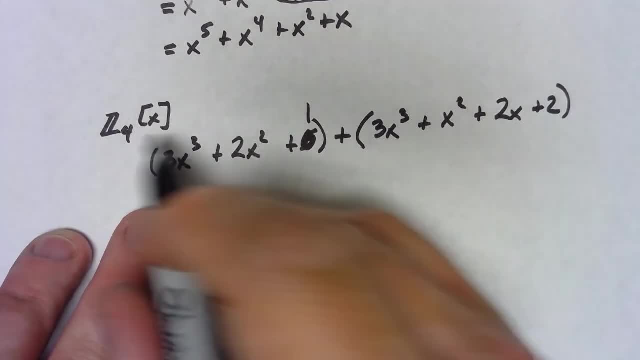 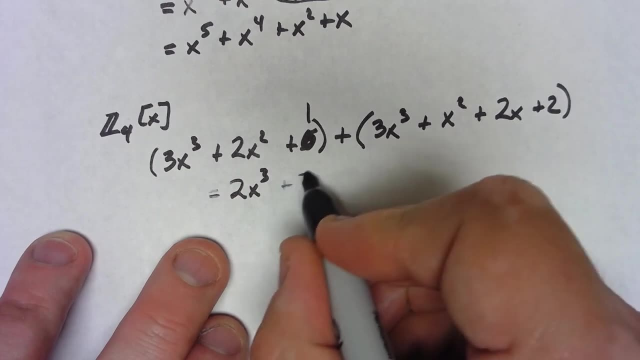 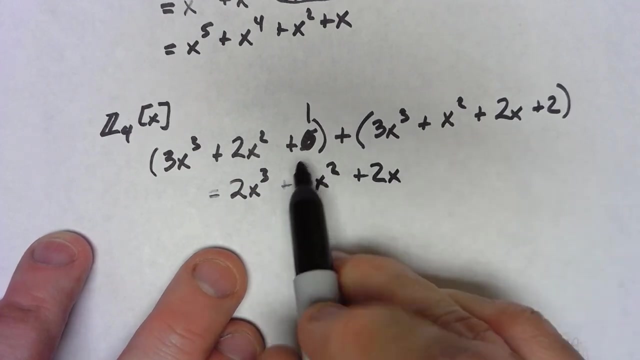 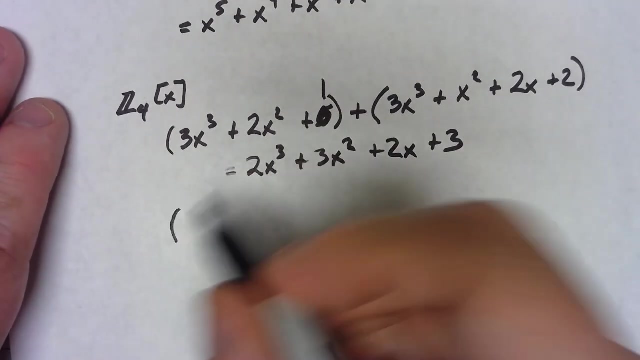 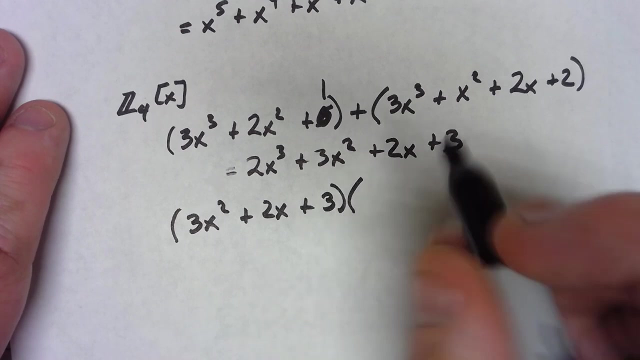 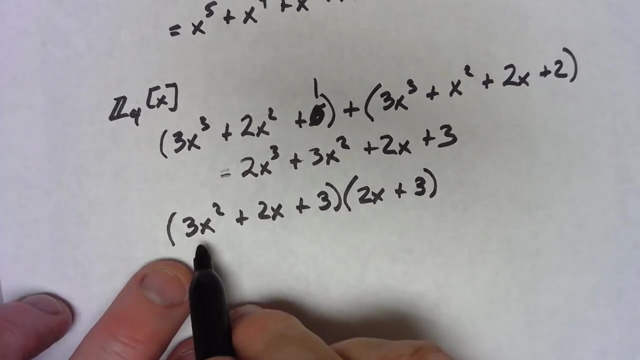 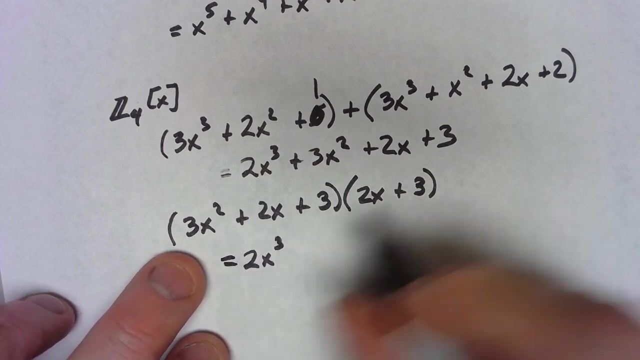 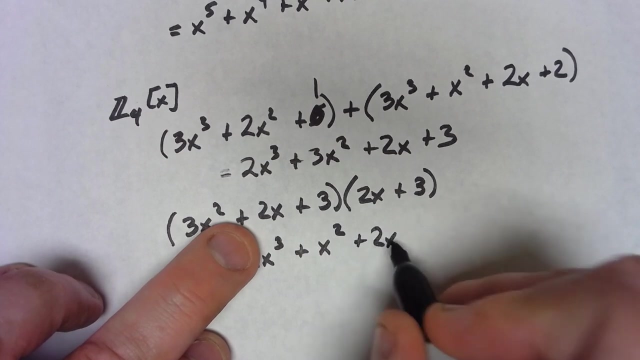 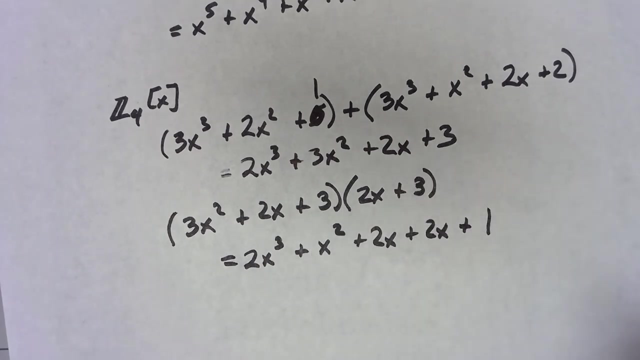 cubed plus 3x cubed normally would be 6x cubed but we've got to do things mod 4 so it's 2x cubed 2x squared plus x squared 3x squared that's perfectly fine there's only a single x and 1 plus 2 gives me 3. all that thing is fine mod 4. If I do 3x squared plus 2x plus 3 times a 2x plus 3 6x cubed would really be 2x cubed we'd have 9x squared would really be just x squared we'd have 4x x squared which is just 0 we'd have 6x which is 2x another 6x is another 2x 3 times 3 is 9 which is really 1.